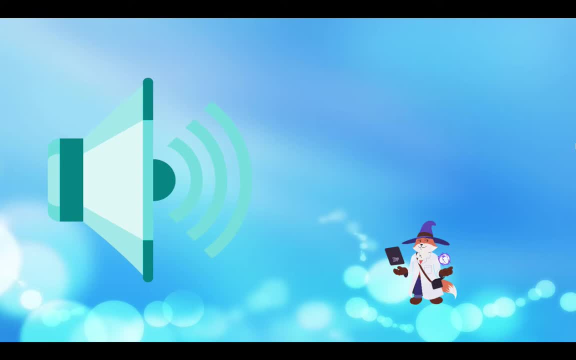 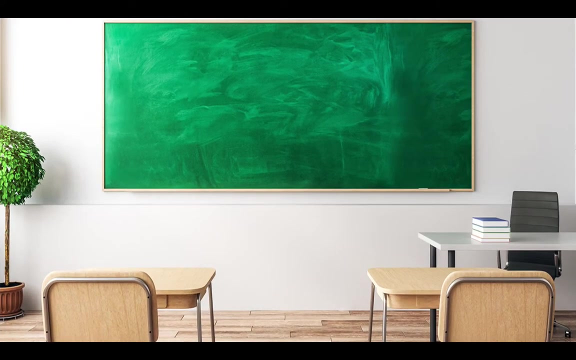 The sound of cars, beeping, instruments playing, the sound of a baby crying or the sound of the door slamming. But how exactly does sound travel? How does sound work And, most importantly, what is sound? Sound has four different characteristics: Frequency, 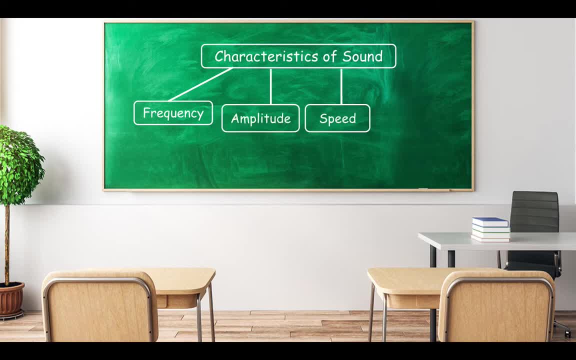 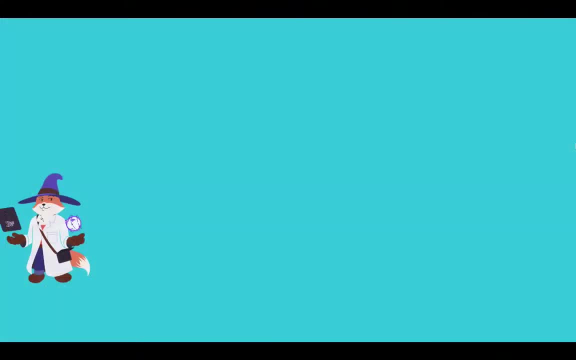 amplitude, speed and wavelength. Frequency is measured in hertz and tells us how frequently an event occurs. To explain it more simply, the more frequency there is, the higher the pitch of the sound is. Let's take a look at this diagram. Frequency means the number of full complete waves passing. 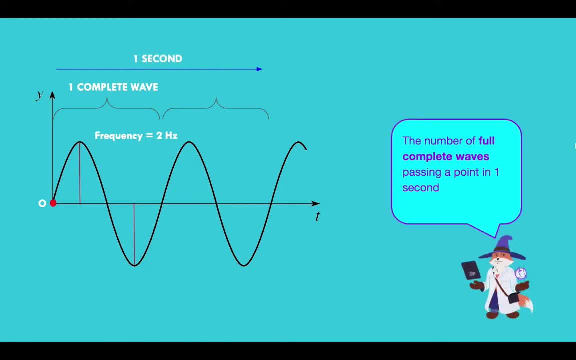 a fixed point in one second. For instance, if one wave is passing point O in one second, then the frequency is one hertz. If two waves are passing point O in one second, the frequency is two hertz. Whoa, it's kind of hard to understand, isn't it? 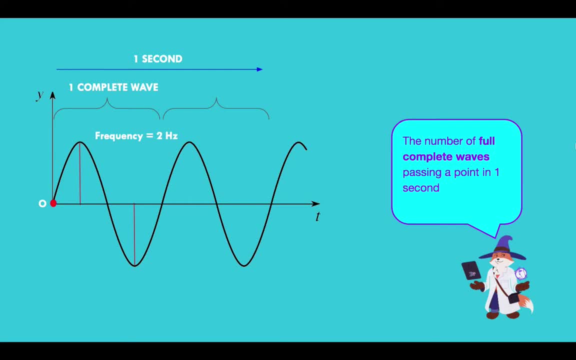 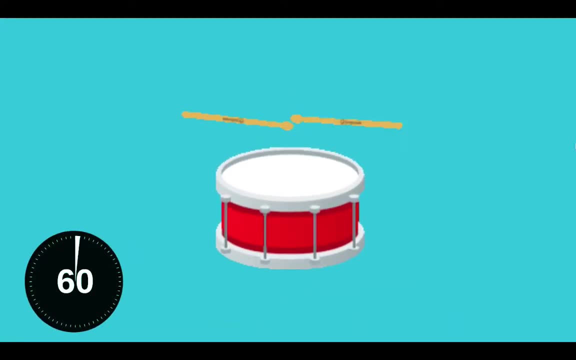 Haha, well, I'm sorry for explaining it too complexly. Now I'll use a drum for a better example. If you beat a drum, with each beat the same speed for one minute and you beat it ten times, the frequency is ten beats per minute. 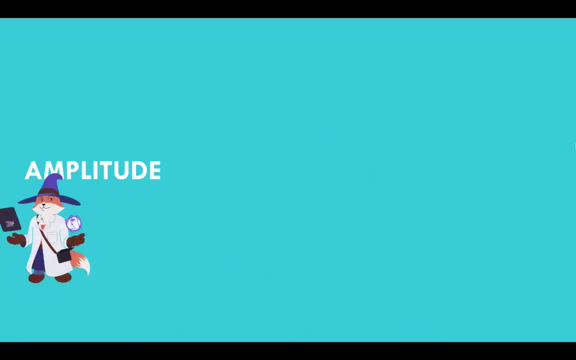 What is amplitude? Amplitude is measured in decibels and simply means loudness. The louder the noise, the higher the decibels. Decibels can also be adjusted to human hearing. According to studies, sounds at or below 70. 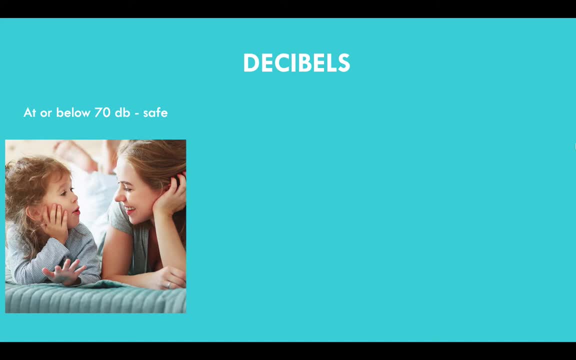 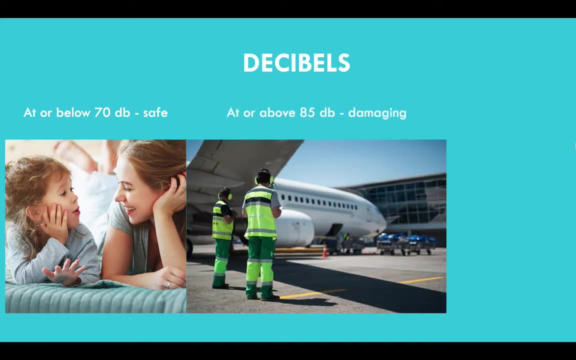 decibels are generally considered safe. An example is the sound of normal talking, which is around 60 decibels. Any sound at, or above 85 decibels is more likely to damage your hearing over time. That's why if you beat a drum, with each beat the sound will be louder. and if you beat 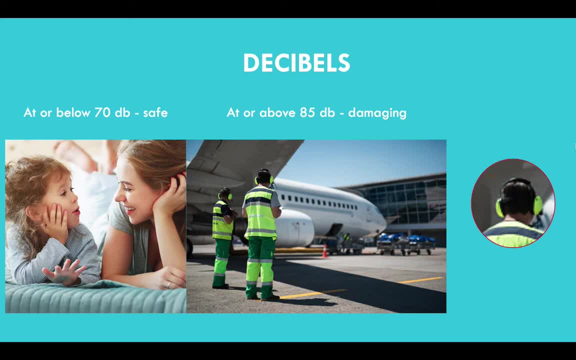 a drum. with each beat, the sound will be louder. That's why airport workers, people who mow lawns and construction workers wear headphones or earbuds at work. On the other hand, the body can also respond to lower noise levels. Sleep can be disturbed. 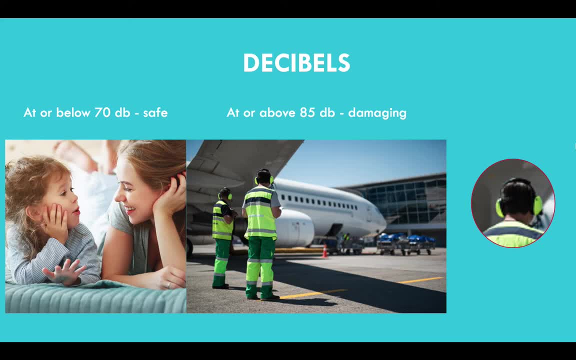 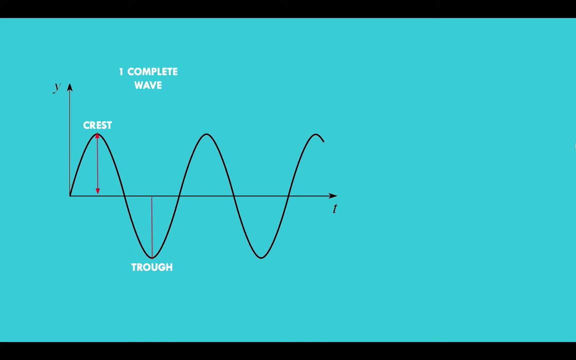 by an outdoor noise of 40 decibels. In this diagram, amplitude tells us the maximum distance of a crest or trough from its undisturbed or rest position. Also, a crest is the highest part of a wave, while the trough is the lowest part of a wave. 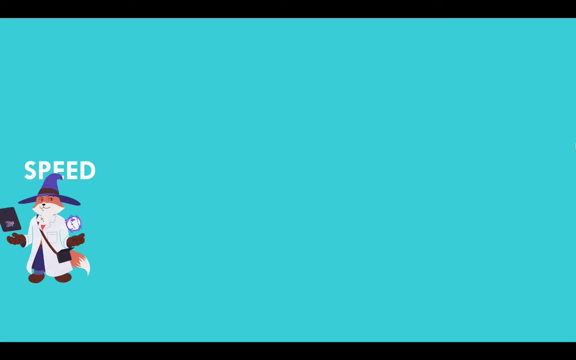 What is speed? Speed is measured in meters per second or other speed measurements. It is the distance covered by a wave in a unit time. My Why do I keep saying things that you don't understand? Fine, so you must know about the speed of a bird flying right. 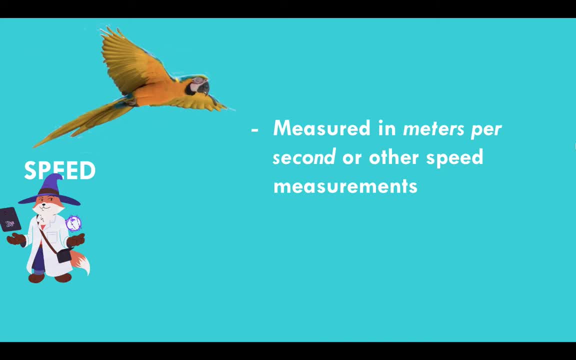 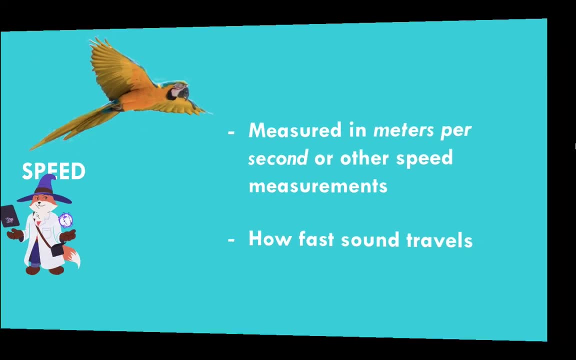 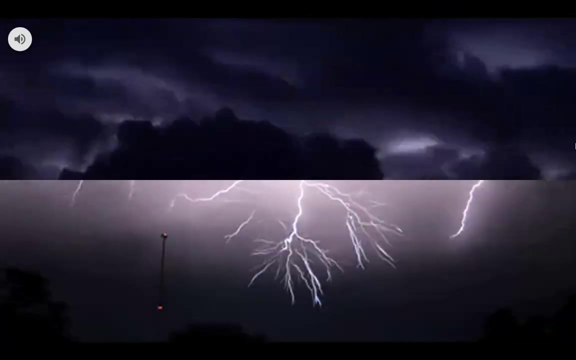 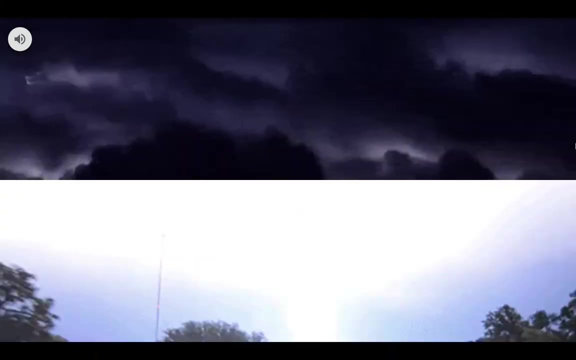 That works the same with the speed of sound. Speed of sound means how fast a bird travels. Let me show you an example. Think about the time when you saw a thunderstorm. Did you hear thunder first or see lightning first? Yes, you see lightning first. 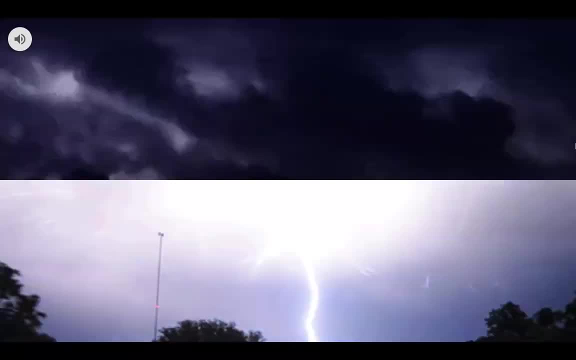 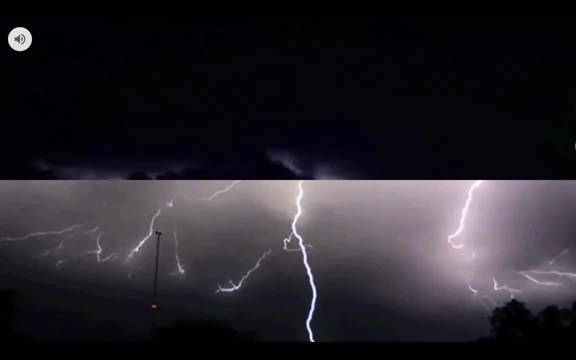 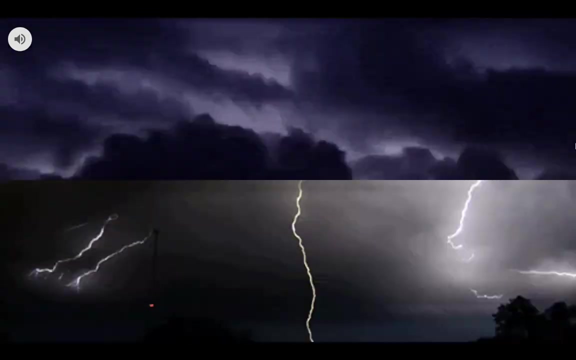 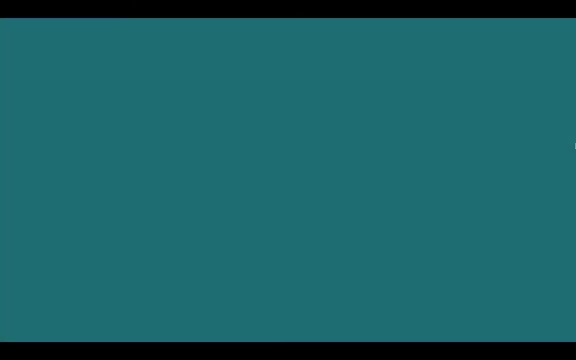 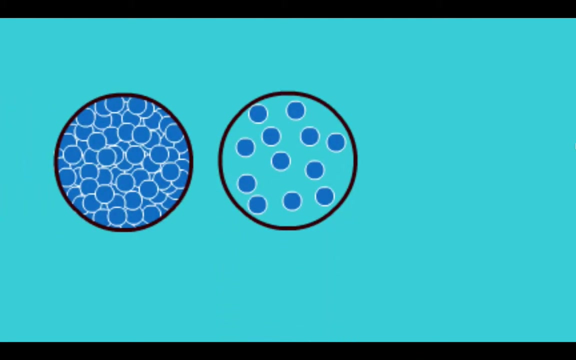 Do you know why? That's because light travels faster than sound. A few seconds later, you will hear thunder. Also, as you know, matter has three states: Solid, liquid and gas. Sound travels at different speeds in different states. 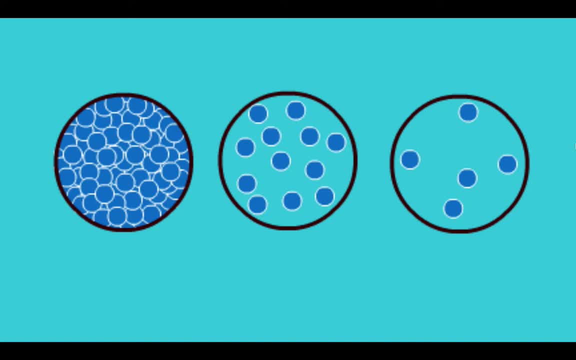 This sounds interesting to me. Here's why Solid objects are hard, which means that they have fixed molecules. Molecules touch each other and stay in the same place, no matter what They are arranged in rows and columns. When sound travels through solid objects, they travel faster. 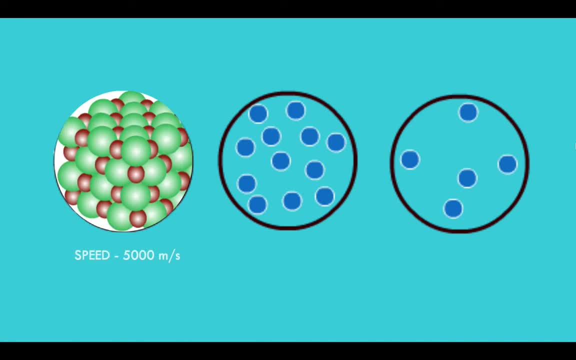 That's why: Because the molecules are touching each other, so the sounds can easily pass through one another. Liquid flows, so the molecules are a bit apart. They move, and move slowly flowing, so the sound passes through slower than in solid objects. 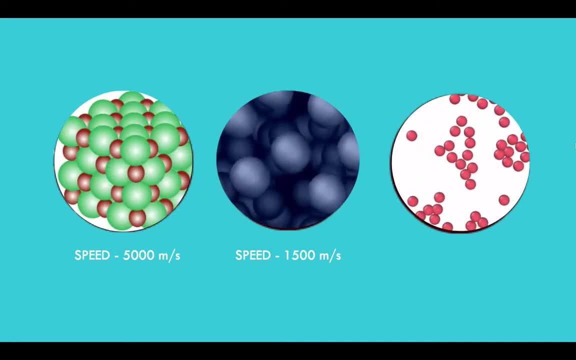 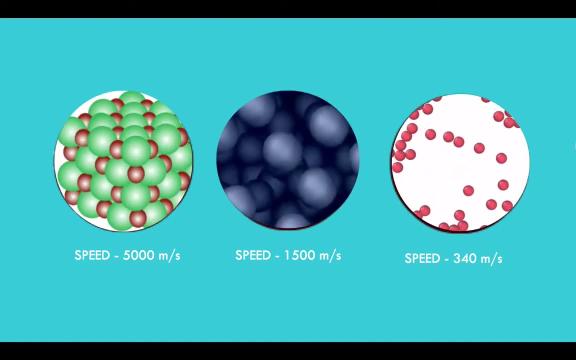 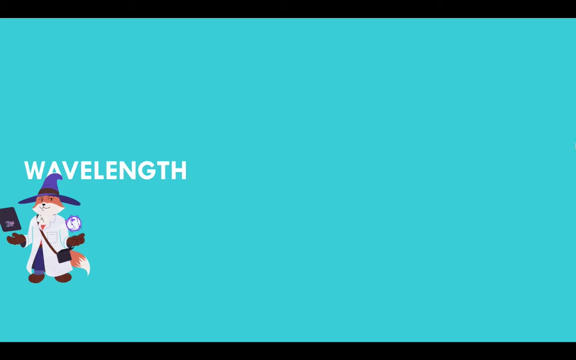 Molecules and gas are far apart from each other and they move fast, causing the sound to pass easily. The sound is even slower. Oh, I think wavelength is much easier to explain. Finally, Wavelengths are measured in meters. It is also working similar to a light wave. 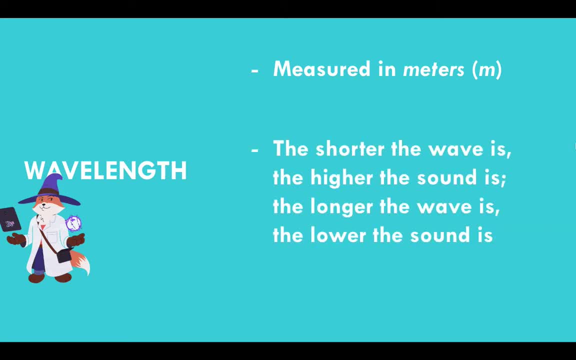 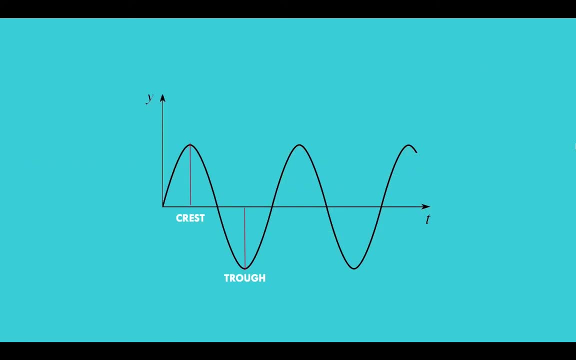 The shorter the wave is, the higher the sound is. The longer the wave is, the lower the sound is. Can you imagine? What do you think? Let us know in the comments. See you next time. Bye everyone. In this diagram, wavelength is the distance between a point on the wave and the same point. 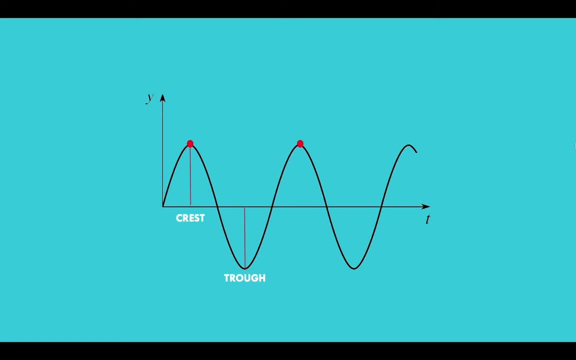 on the same side of the next wave. The two points can be located in the crest of two waves or in the trough of two waves. Well, can humans hear all sounds in the whole wide world? Great question. but no, of course not. 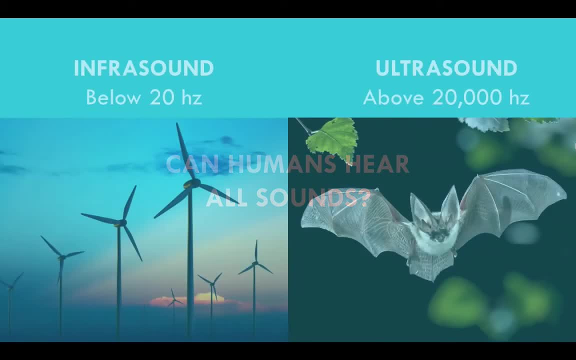 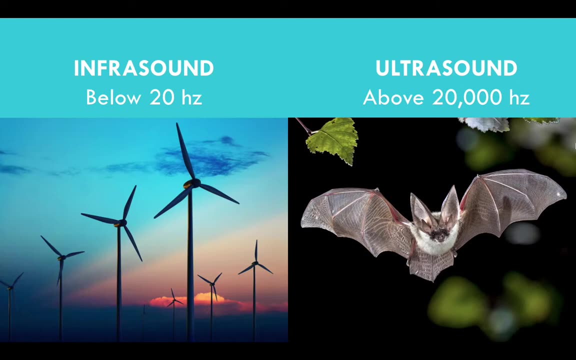 Let me explain. Any sound below 20 Hz can be considered infrasound. Infrasound is sound humans can hear. One example is the sound of a car, The sound of an electric windmill spinning. Sounds above 20,000 Hz are called ultrasound, which we cannot hear. 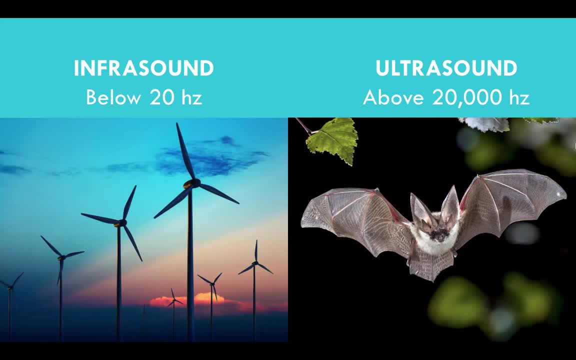 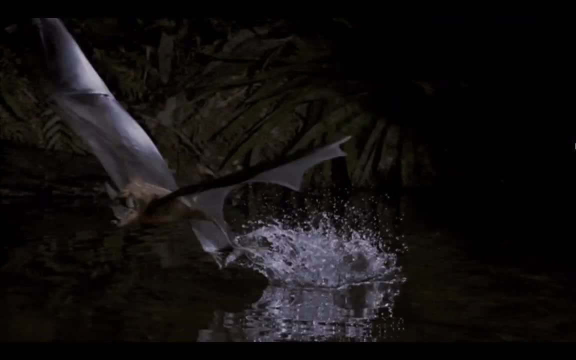 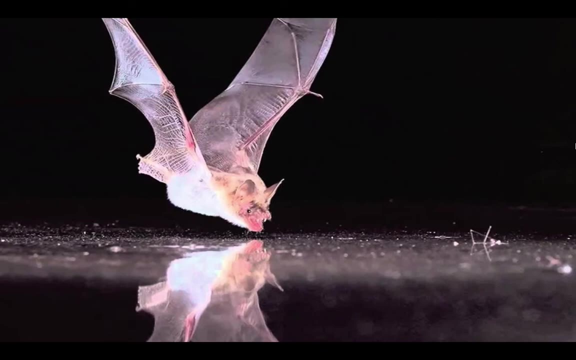 Did you know that ultrasound that we cannot hear is super useful to humans and animals? One example is that bats use ultrasound to find insects or prey in the dark. How does it work? The ultrasound hits the prey and bats expect to hear it. Then it can hear the sound of the snake. 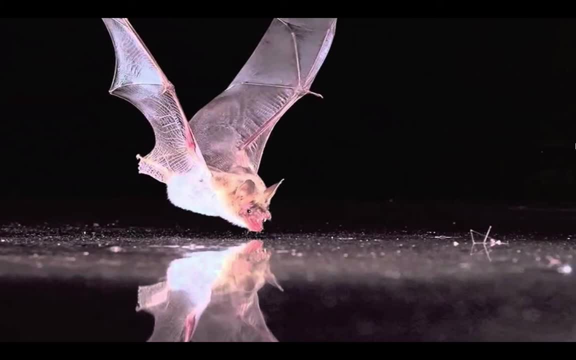 The sound of the snake is the sound of the snake being bitten by the snake. It also listens to the sound of the bat, and then the sound of the bat follows the sound to find its prey. This is called echolocation. Without it, bats would starve in the night. 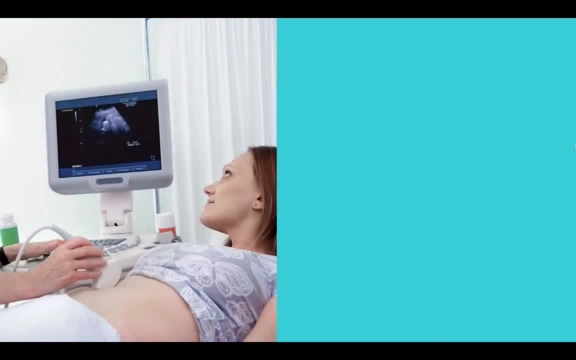 Another example is that ultrasound is used by doctors to scan unborn babies inside their moms. It is used to check if the babies are healthy and normal. The results appear on the screen. We have a sonar styled, pixelated ultrasound. We can also see a sonar box. 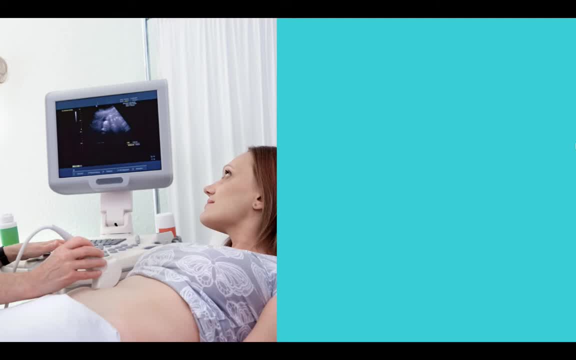 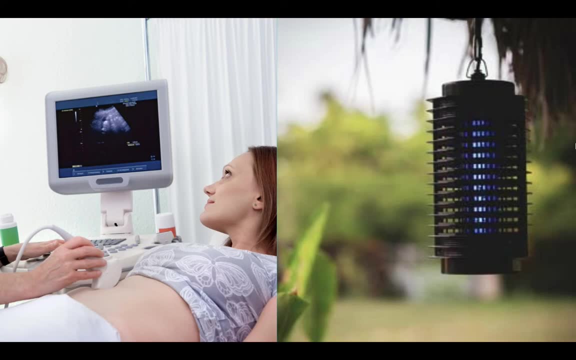 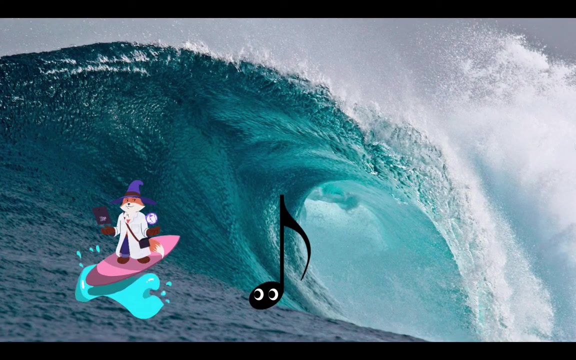 picture of the baby. Ultrasound is also used to scare away pests from our house. Rats and insects can hear ultrasound. It is a horrible sound to them, so the possibility of pests in your house will immediately decrease. So we have just discovered how interesting sound is, even though it seems like a normal. 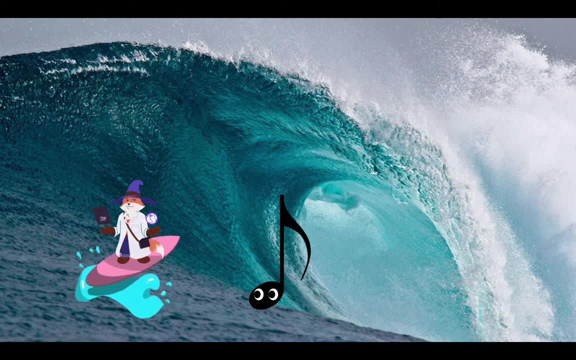 thing to hear every day. There are sounds you cannot hear, and sounds that can also be measured in waves. Oh wait, oh hi, musical note. Hi, Professor Mega, Let's go surfing together. Sure, I'll get you a surfboard. 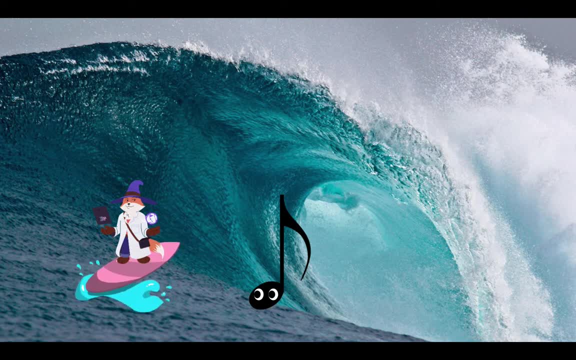 Okay, Be careful of the ocean waves. Oh, I mean, I'm not surfing on an ocean wave, I'm surfing on a sound wave. Oh, come on, I cannot even do that. We'll try Here. Ah, Oh, are you okay? 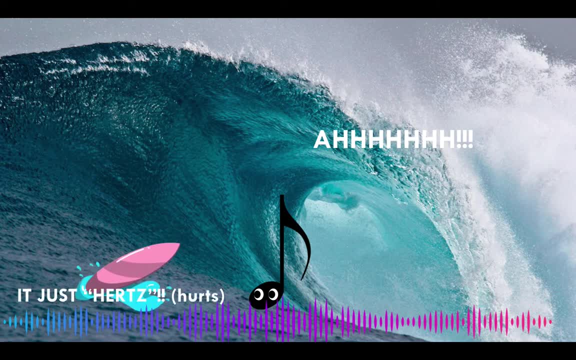 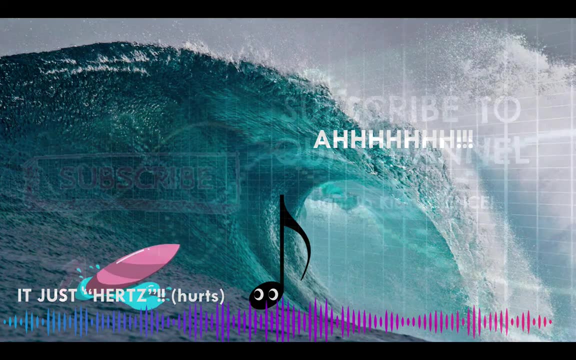 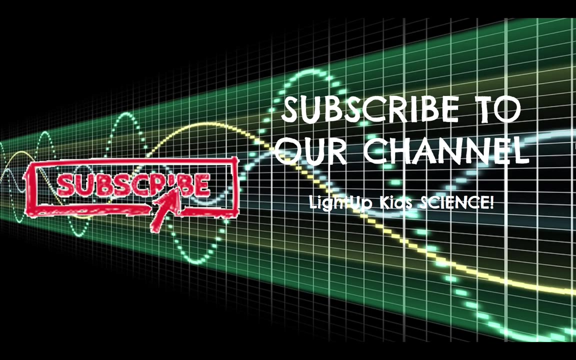 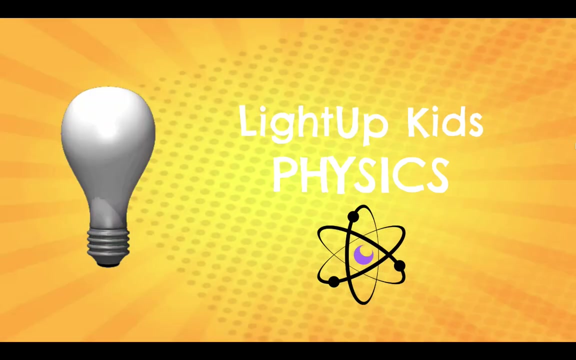 Yes, but it just hurts. Subscribe to our channel. Light Up Kids Science. Light Up Kids Physics. 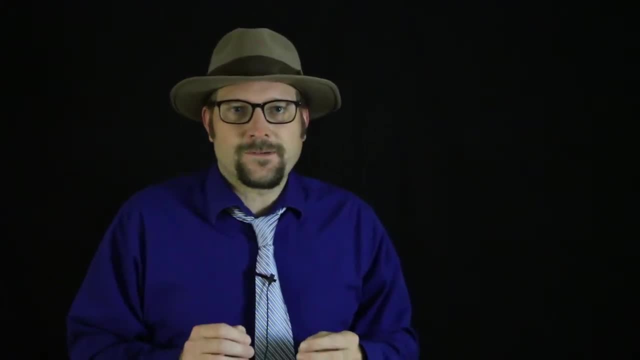 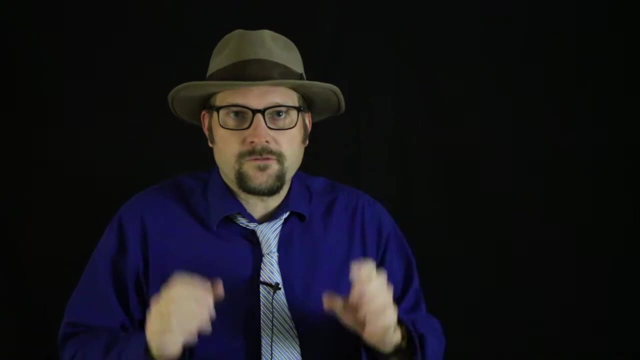 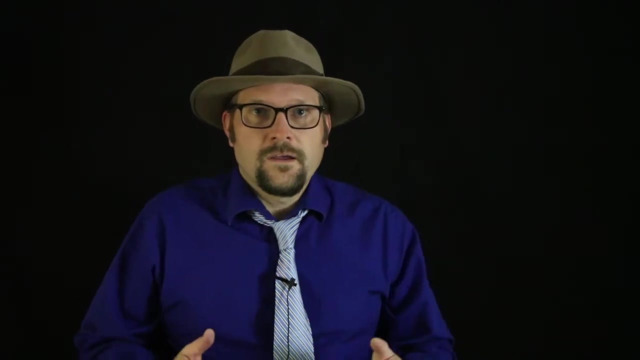 Welcome to Utah State University's Vertebrate Paleontology course. My name is Benjamin Burger and in this lecture I will summarize the three major groups of Triassic archosauromorphs. The first group of basal archosauromorphins from the Triassic period are the Protosauria.